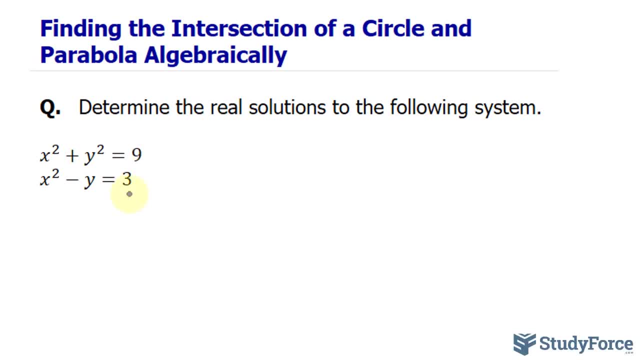 This 9, if we square root it, we get the radius for that circle. The second equation is: x squared minus y is equal to 3.. If I rearrange this formula and isolate for y, I end up with a quadratic. I know it's a quadratic because x is being raised to the power of 2.. 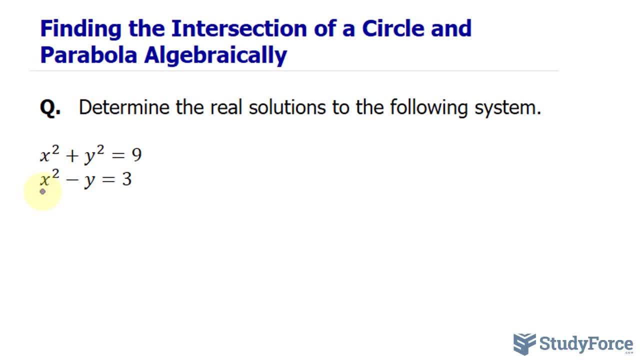 And that, of course, forms a parabola when graphed. Now there are several ways that you can find the solution to this system of equations. You can use substitution, which involves isolating for one of the variables and then substituting it back into the other equation. 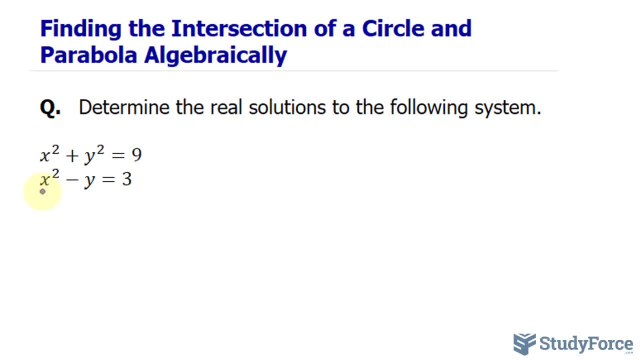 And the second method involves elimination. Elimination is when you eliminate one of the terms so that the resultant equation has one variable only. I think the easier of the two methods for this in this particular example is substitution, And I'll start with equation 2, the second equation. 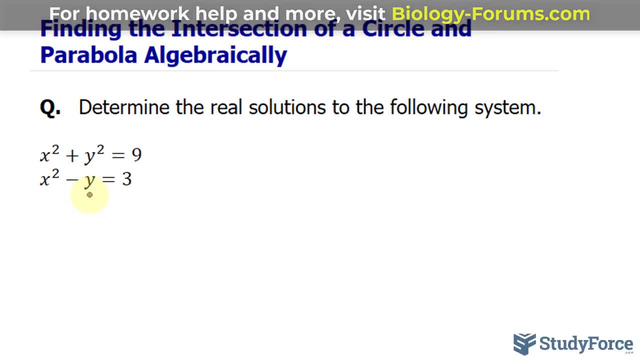 Let me go ahead and solve for x squared. I know that's a little unconventional, but if I solve for x squared by bringing this y over, I end up with x squared is equal to 3 plus y. The reason why I've chosen to do this is because 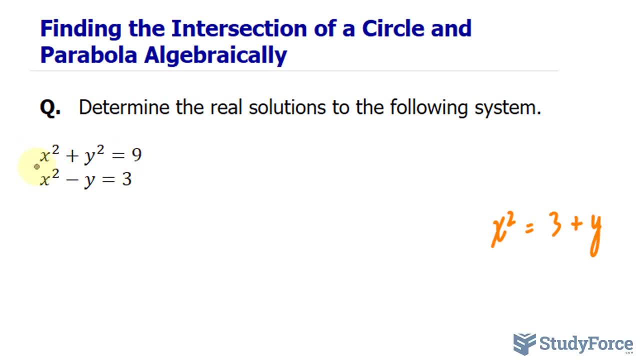 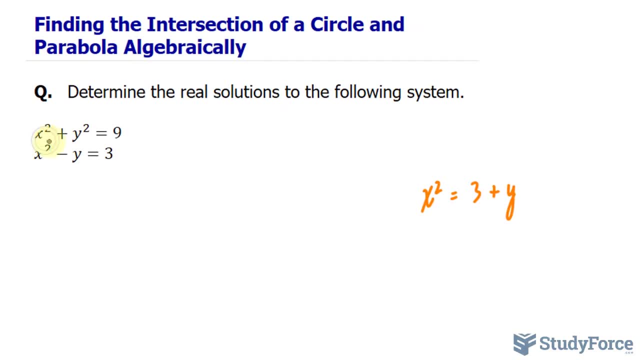 notice that in this equation we have an x squared term and I can replace that x squared term with 3 plus y. Let me show you why that is a good thing. So replacing x squared with 3 plus y, and then the rest of the equation is plus y squared- is equal to 9.. 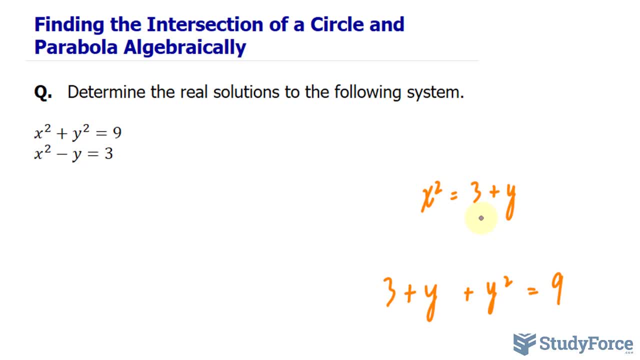 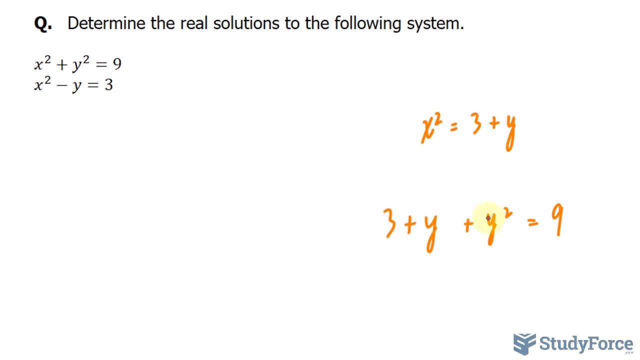 As you can see, by replacing x squared with this expression, we now have a new equation that is exclusively in terms of one variable, in our case y. So I'll go ahead and solve for y in this equation, which is a quadratic. 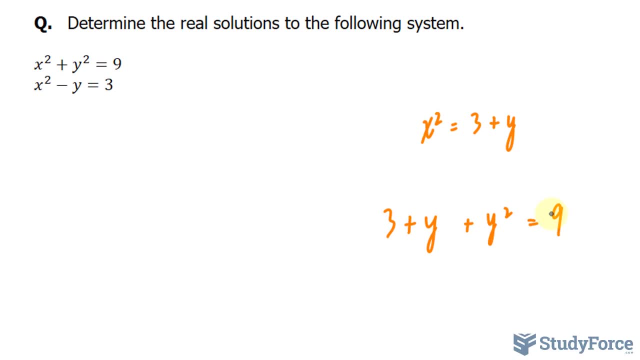 It's a second degree equation. We have y to the power of 2.. I'll bring all the terms to one side and notice that this 9 is on the right side. I'll take it to the left side as well, where I have y squared. plus y plus 3, minus 9 is equal to 0.. 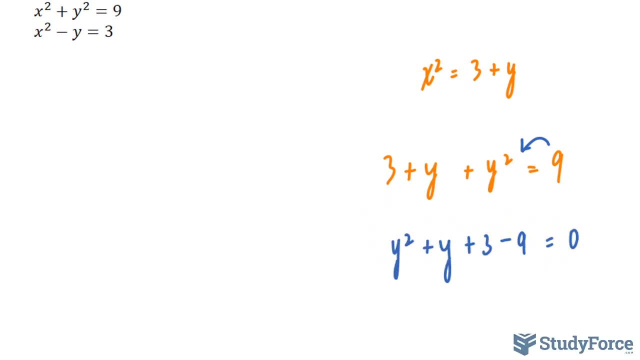 I just rearranged the terms so that the highest degree term is at the front. 3 minus 9 is negative 6.. y squared plus y minus 6 is equal to 0. And luckily for you, this can actually be factored through trial and error. 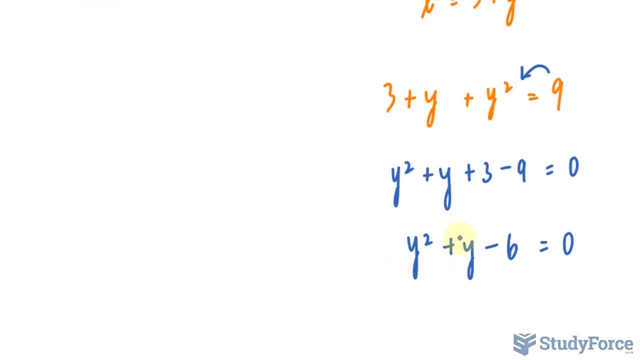 What two numbers multiply to negative 6 and add to positive 1? The two numbers that come to mind is positive 3 and negative 2.. 3 times negative 2 gives us negative 6,, which is this constant term, And 3 plus negative 2 gives us positive 1,. 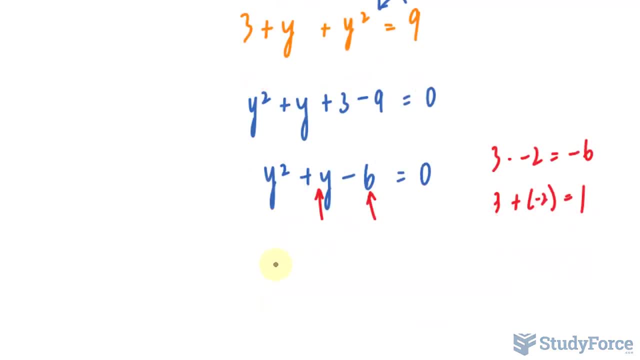 which is the coefficient of that term. I'll break this down into factors: y plus 3 and y minus 2 is equal to 0.. Solving this equation now we get: y is equal to negative 3 and y is equal to positive 2.. 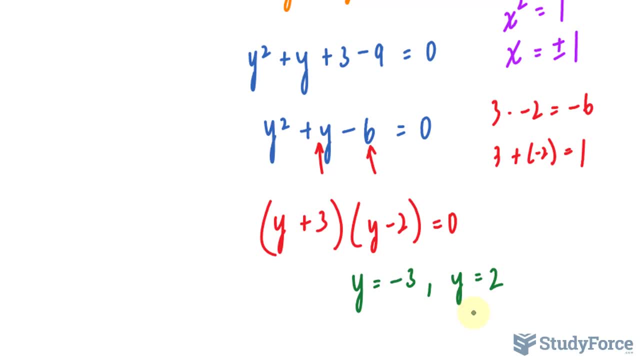 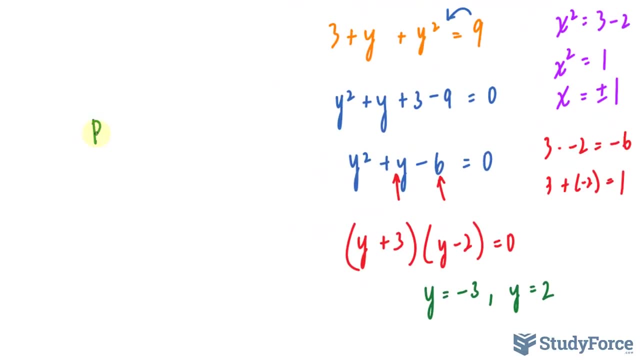 These y's that we found could potentially be the y-coordinates of points that represent the intersection of these two equations. So I could potentially have a point 1, that has an unknown x value, which we've yet to find, and the y-coordinate negative 3,. 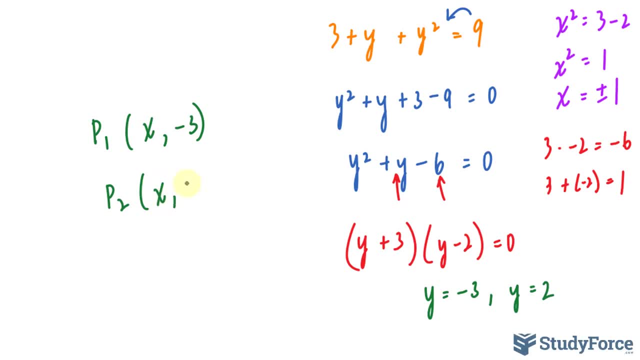 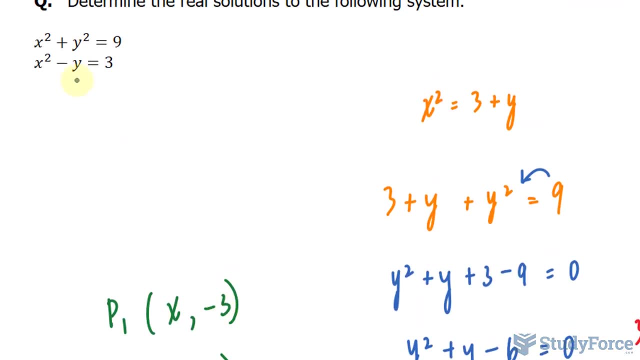 and a second point: x and positive 2.. To find out if these are actually points or y-coordinates to points, I'll take this negative 3 now and substitute it into here. Let me show you what I mean I have: x squared is equal to 3 plus negative 3.. 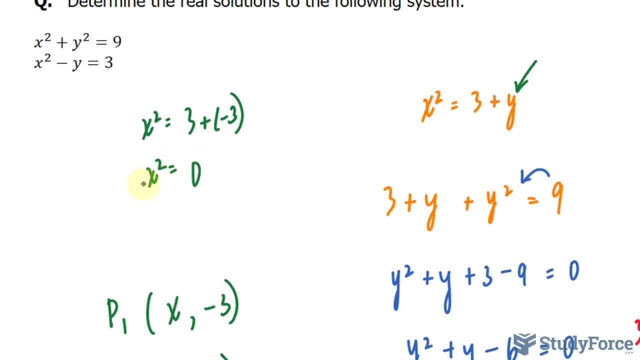 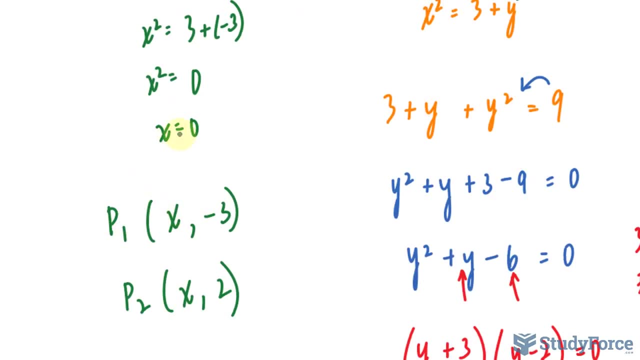 The right side combines to 0. We have x squared square root of both sides We get x is equal to 0. This means that the x-coordinate of this point is 0.. For point 2, I'll take this 2 now. 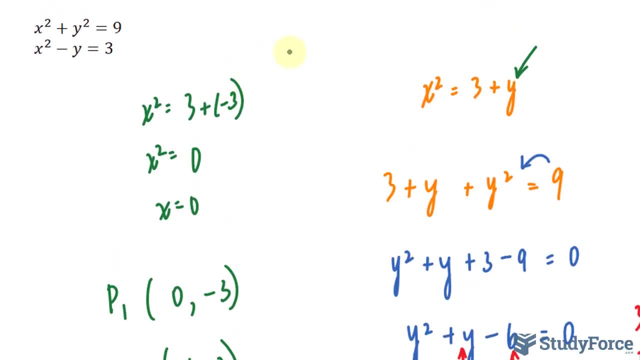 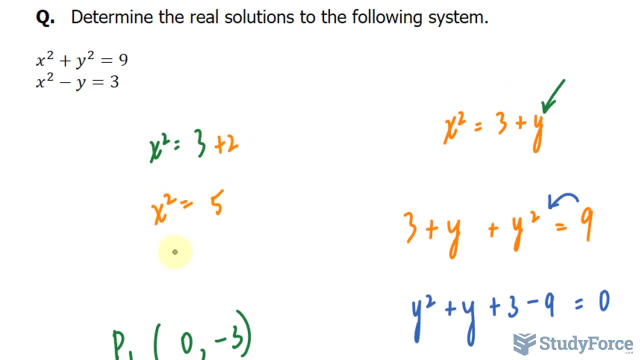 and give it the same treatment as that negative 3.. I'll throw it into this equation: We have 3 plus 2, and that combines to 5.. Square rooting both sides we get x is equal to plus minus the square root of 5.. 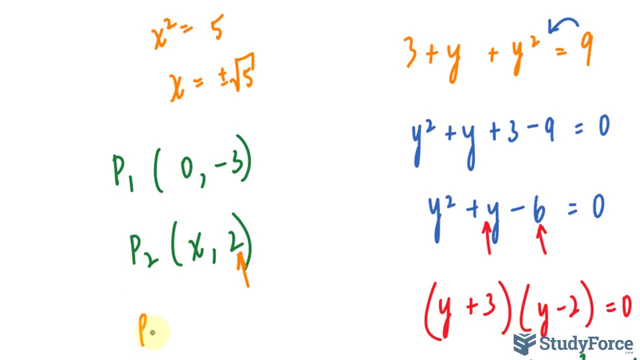 That means we actually have 3 points of intersection. We'll have even a third point where the y-coordinate is 2, and the x of this one will be the square root of 5, and the x-coordinate of this one will be minus the square root of 5..